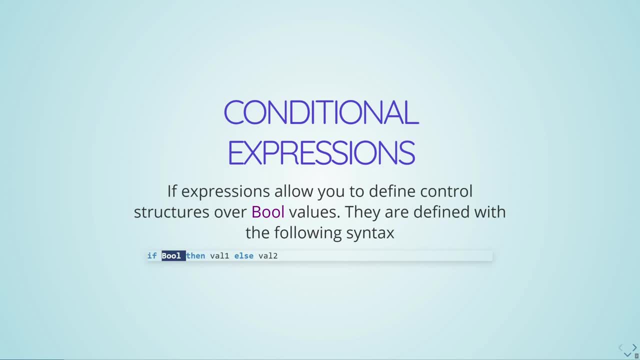 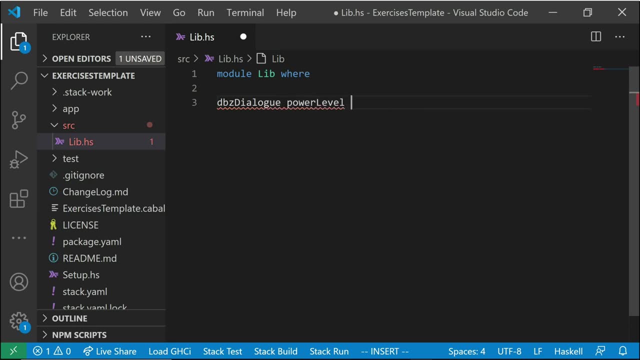 it will return val1.. If it's false, it will return val2.. Let's work through a little example. Let's create a function here And it's going to take an input- power level- And we say: if power level is less than 9000.. Okay, so this will be our boolean expression here. So this is going to 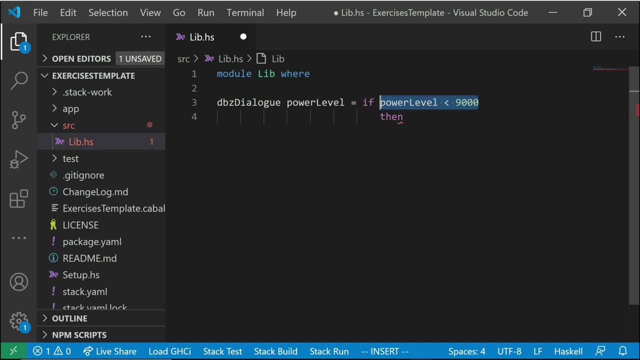 return either a true or false boolean expression, And if it's true, it will return val1.. And if it's true or false value, if we didn't put a boolean expression here, like, let's say, we just put 9000 here, this would be an error. we can't do this, So we need to return. 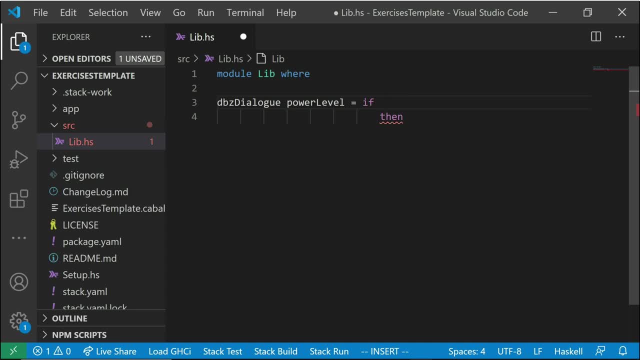 some sort of boolean expression inside this level. Okay, if it is less than 9000, then we'll return some expression. So let's just return a string here, lame Else. if it is over 9000,, well, it's over 9000.. Need a number of exclamation marks here. 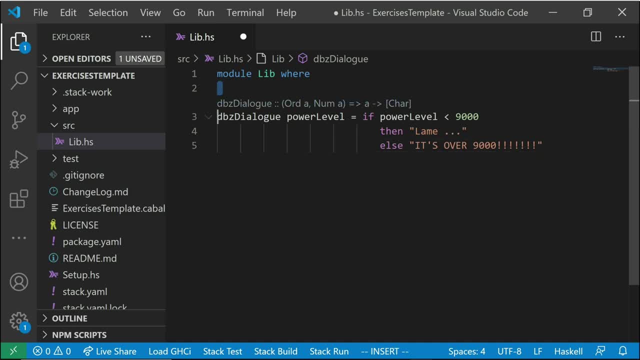 Okay, and the type of this function, ignoring the default type that's trying to give us here, which is a bit more complicated than it needs to be, is going to be the dialog. Let's say, power level is an integer that's suitable. So we're comparing it to 9000.. Okay, so, 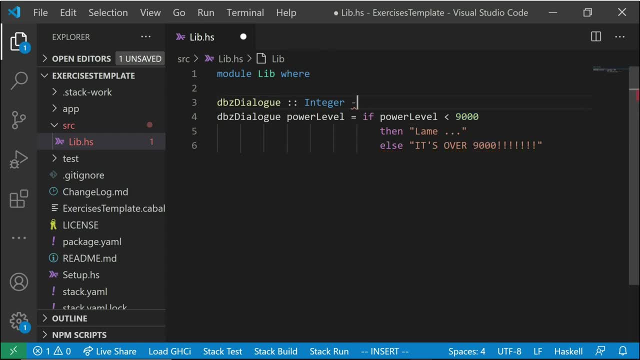 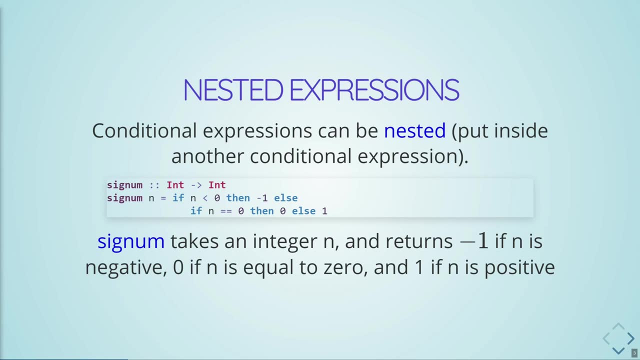 we use, that will be suitable, saying it's an integer itself And it's going to return a string. An interesting thing we can do with conditionals is nest them inside of one another, So this allows us to create multiple layers of control flow. So take, for example, the function signum, which 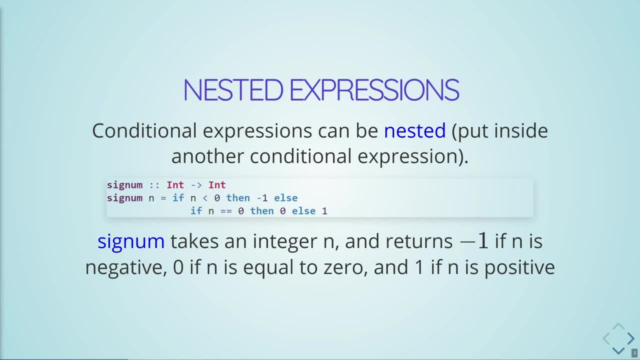 returns negative, one if the int given to it is a negative number, zero if the int is zero and one if the int given to it is a positive number. So usually a just a standard. if can test one condition and then on that condition give two different possible answers, Okay. so you'll notice that. 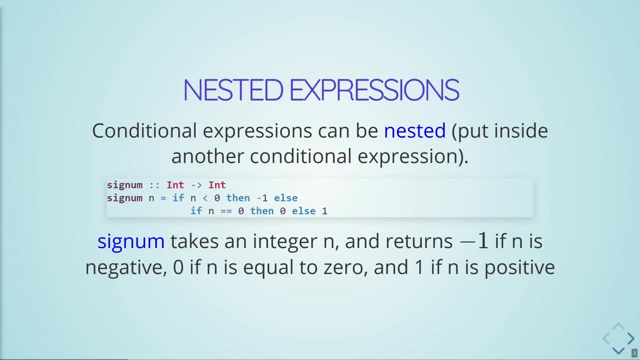 in order for signum to work, there's three different possible answers, three different scenarios that it can return here. So we're going to need a extra if inside of the initial condition. So we'll. we'll start off by testing. Is it smaller than zero? If it is, then it's negative one off the bat. Okay, then we just 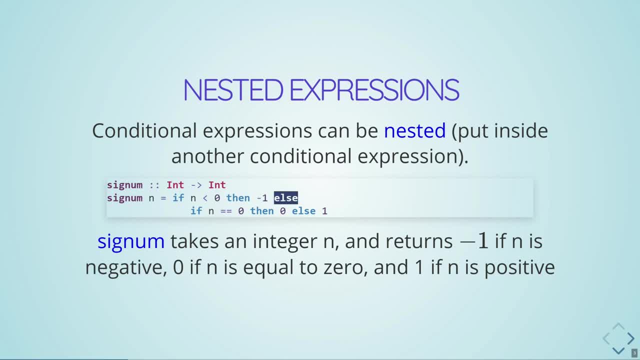 forget about everything else. If it isn't smaller than zero, then we have to have an else here, And then this else is a whole, nother conditional expression. Okay, so this is. you could consider this whole expression that I've highlighted here to be wrapped in brackets. Okay, so this is a. 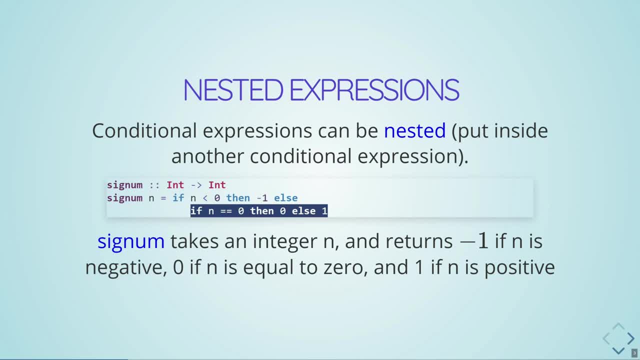 whole nother expression. that gets evaluated and then it tests: is n equal to zero? Okay, if it is equal to zero, then it's just a negative one. Okay, then we test. if this is a negative one, we return 0, else we return our final expression. It is important to note when: 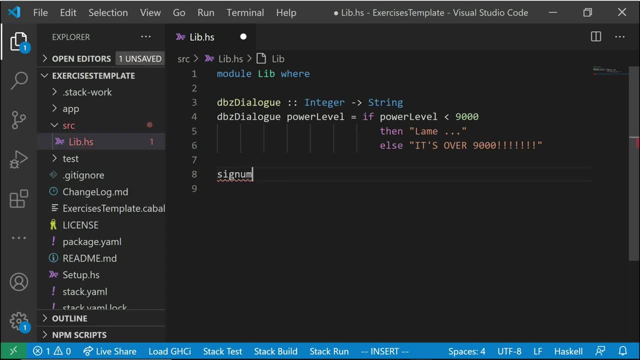 writing if expressions. indentation is important. I brought this up last tutorial, but just a quick reminder. you could write the whole if expression on one line. so you could just write everything as on one line. say: if and small equals 0, then negative 1, else and equals 0, then 0 else 1. okay, but this: 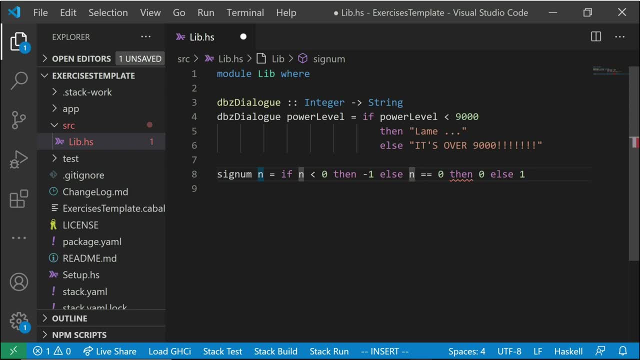 starts to look pretty messy and actually made a little error here. so you'll see it, even notices it right away. it says parse error. so parse error is like well, something's not right here, just right off the bat. it's not gonna compile, so you'll notice I am missing in my else here. if there we go, okay and so. 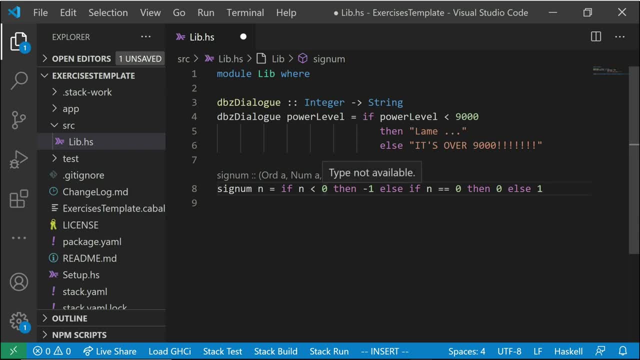 I could write this all on one line, but doesn't look very good, right? usually, when a I write an if expression, I'll say: if I'll write you, you, you, my conditional, okay, my Boolean expression there, and then I'll start a new line and I'll indent. 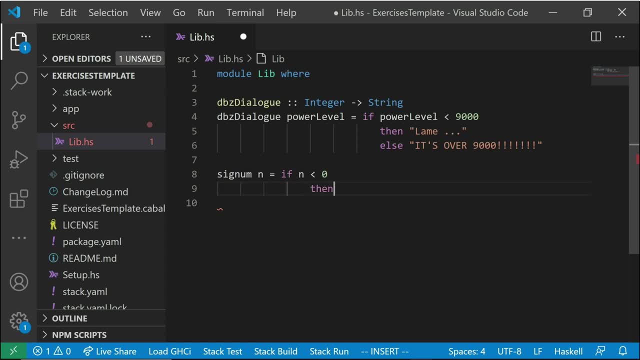 inside of the. if so, I'll indent a bit further in and then I'll write my then. okay, so if it's smaller than or equal zero, then negative one, and then I'll make a new line again and you have to. 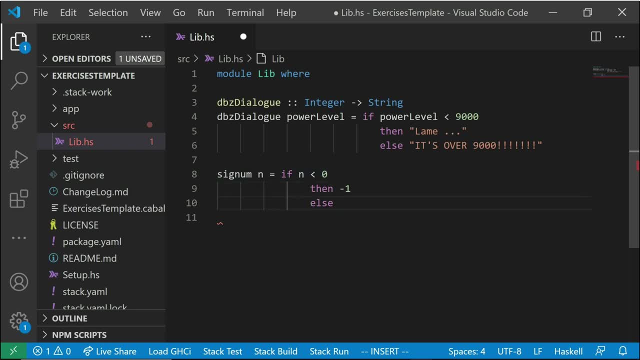 make sure these line up, the then and the else line up here. okay, make sure they're on the same line here. and you're gonna have to be careful if you're mixing spaces or tabs. okay, back to the spaces versus tabs debate. okay, if everything is always spaces all the time, you won't run into. 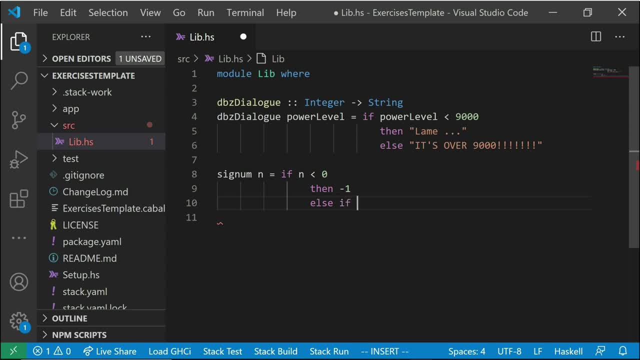 some issue here On the else here. now I could write my next if expression. I'm going to do the same thing, I'm going to say, okay, else, if n is equal to zero, then okay. so now this then: 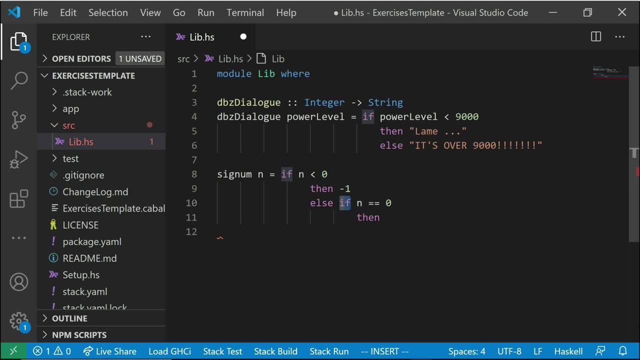 now has to be indented from this. if you have to keep track of which, then belongs to which. if okay, so then zero, else one. So this is all one expression here And this is all one sub expression to this expression, So I can actually put brackets around this thing. 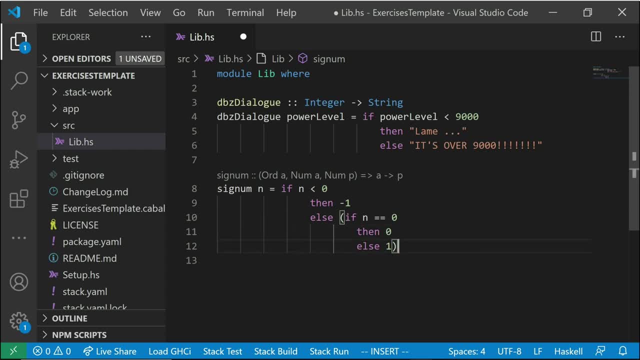 Just to be ultra specific about what's going on here. Okay, so with or without the, if the brackets the same, the same sort of precedence, that's happened. okay, But the brackets just emphasize what is happening here. So this is all one sub expression, that is the. 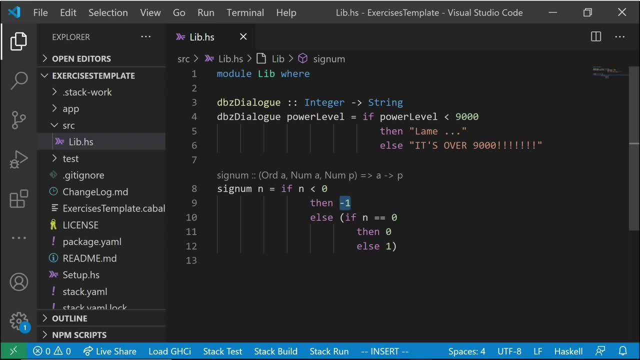 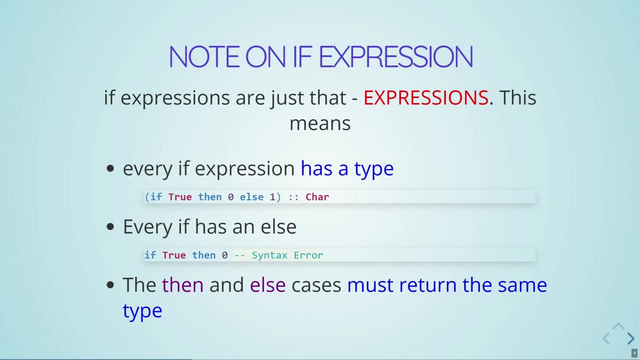 expression that gets returned by the else. the same way, this negative one is the expression that gets returned by the then. Now a note on if expressions in Haskell, if expressions are just that: expressions. So what does this mean? So every expression is going to have 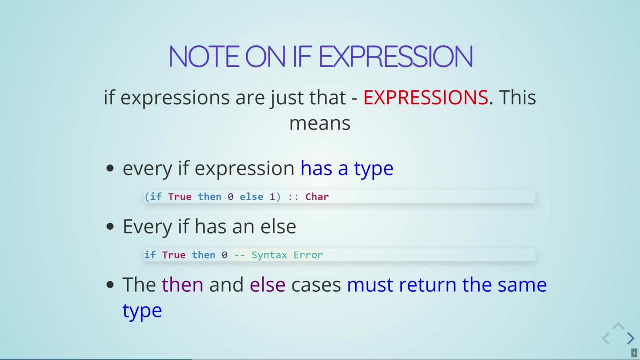 a type. So the idea here is, if you think about expressions as like the expressions you're probably used to from math, they all kind of evaluate to one value, okay, and that value is going to have a type at the end of the day. So an if expression, it's going to evaluate to one value. 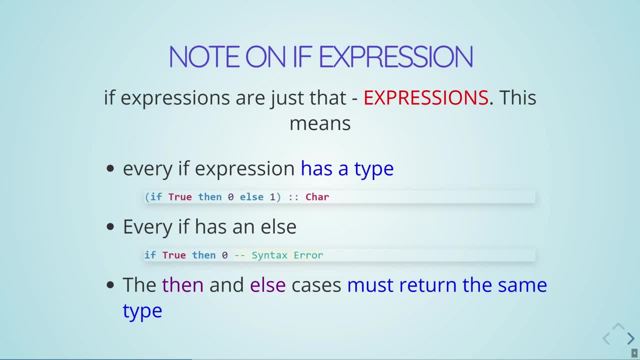 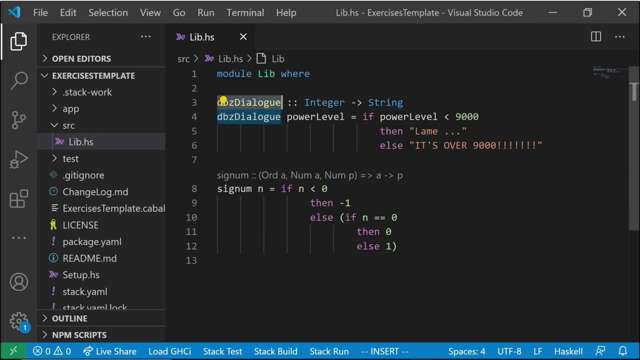 at some point and that value is going to have a type. So let's take a look at our functions here. So let's go back to our function. So this DBZ dialog: it returns a string. Okay, so this is relying on the fact that this- if 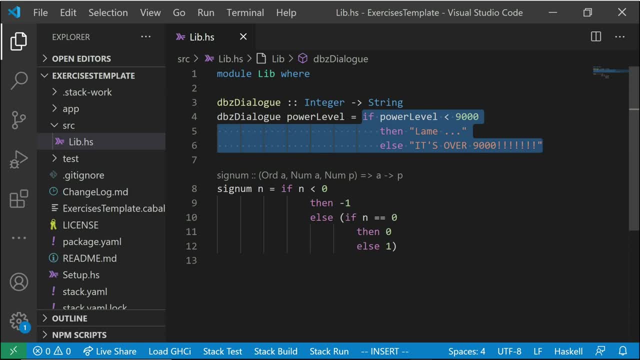 expression it's going to evaluate to a value. okay, just like, how you know, one plus one minus two, any math expression. eventually it's going to evaluate to one value. okay, In this instance, that would evaluate to zero, right? And so this is going to evaluate to one value. 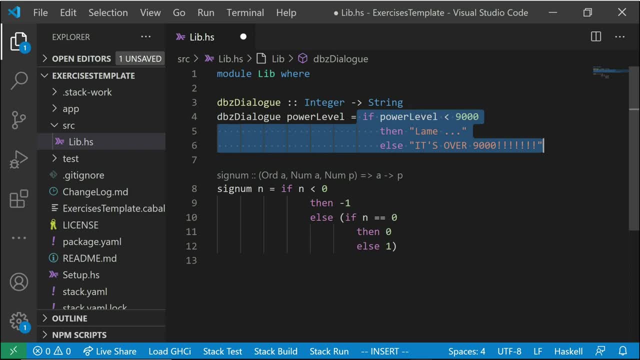 okay, at some point there is a control flow Here, So there's a decision on exactly what that value is going to be. But when it does evaluate to that value- whatever that value is, that it's going to have to have type string. So if I were to 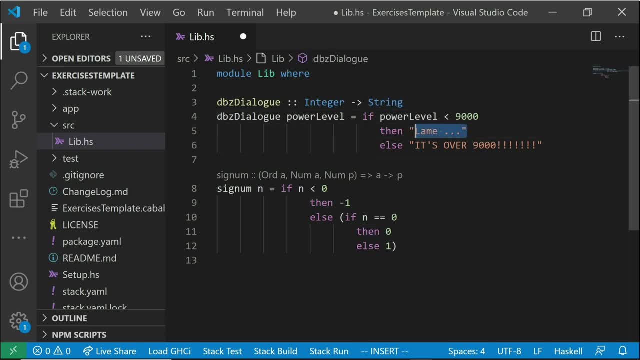 switch this up and say: Well, if it's under 9000,, then I return zero. This is a type error, okay, Because now we have one situation where this function returns an int and another situation where this function returns a string. this can't be. this function has to return one type, Okay. so 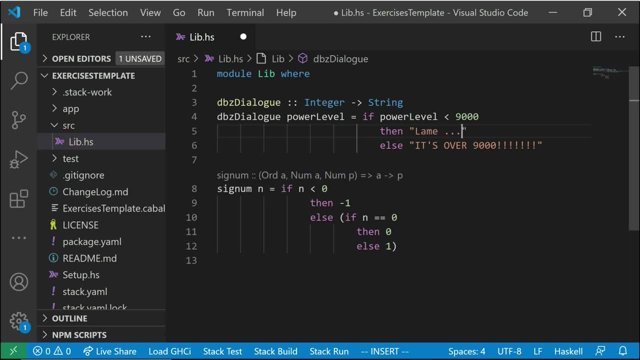 we can't. we can't just switch things up willy nilly, returning one type at one time and another type at another time. Same with signum here. Okay, so if we add the less complicated type, then what VS code is suggesting? we could say, well, signum. 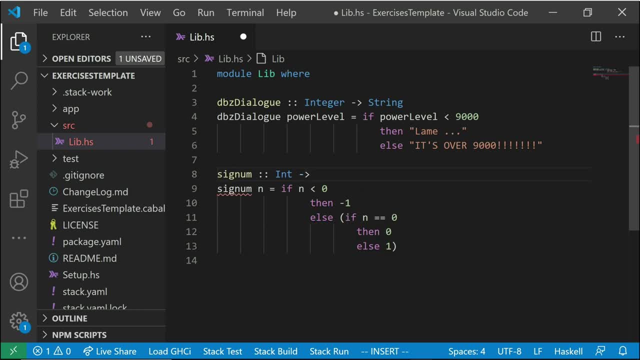 takes an int And a returns a another int. Okay, so I can't magically say: well, if this is less than zero, then we return It's negative, we return a string here. Okay, this is also a type error. Okay, and 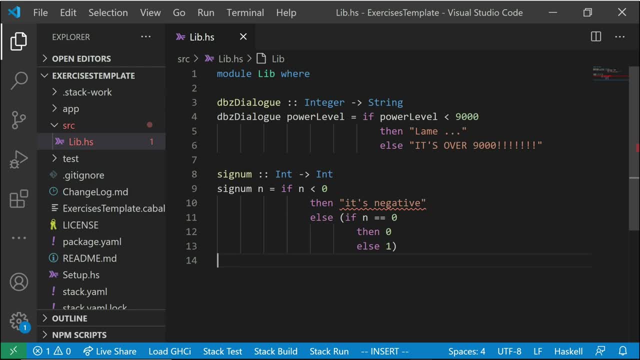 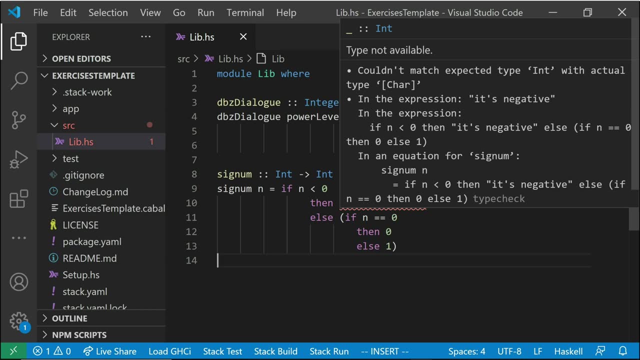 we can. we can put our mouse over this, So see how it's underlined red. if you put your mouse over it, this will appear and it'll tell you the type error. So it's the general. couldn't match expected type, So it was expecting an int, but it got a char, Okay. 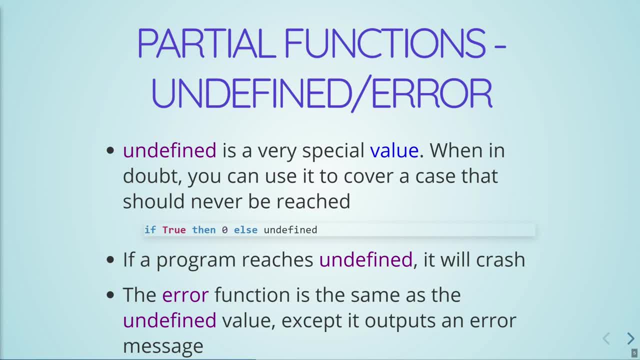 The one exception to what I just discussed is partial functions. So basically, anytime, instead of returning a value you've returned, you can consider this a special value called undefined. So, at any point in time, instead of returning a value of a specific type, you just say undefined, And what actually happens is when. 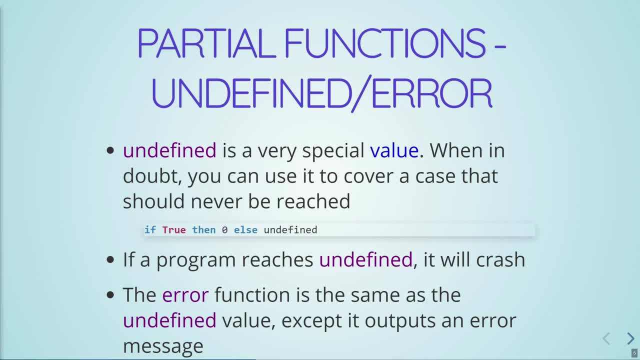 Haskell is evaluating stuff and it runs into this value undefined. it just crashes. Whenever it reaches undefined, the program will just crash. Now, undefined is actually available, so you could just write undefined in your code, but it's better to use the error function. 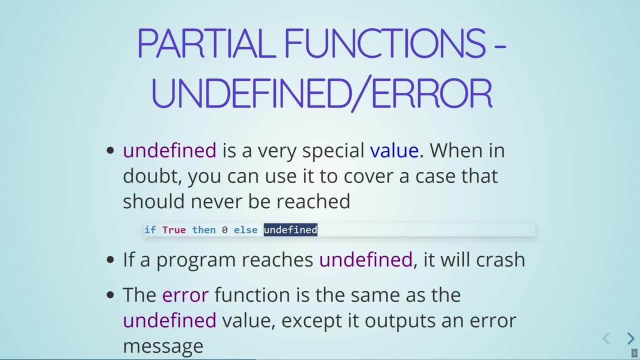 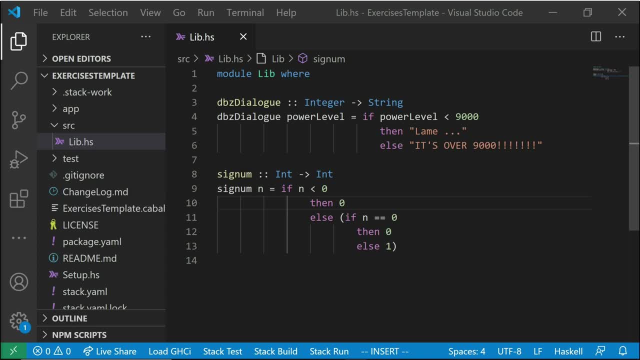 which is the exact same thing as undefined. However, it outputs a specific error instead of just saying reached undefined. As an example, let's say when powerLevel is less than 9,000, instead of returning a string, we just write undefined. 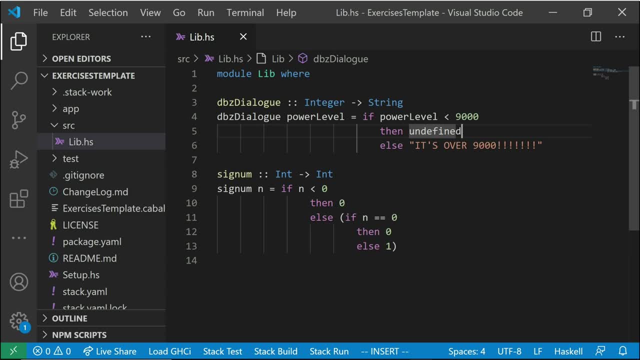 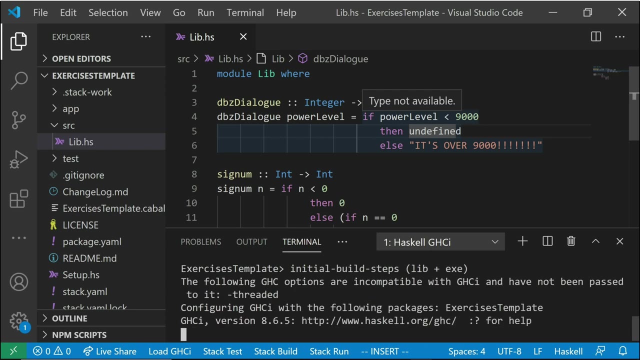 So we just let our program crash. So if the powerLevel is not greater or equal to 9,000, then there's no point in this. We should just crash. the program should just die. So if we load this into GHCI to test it out, 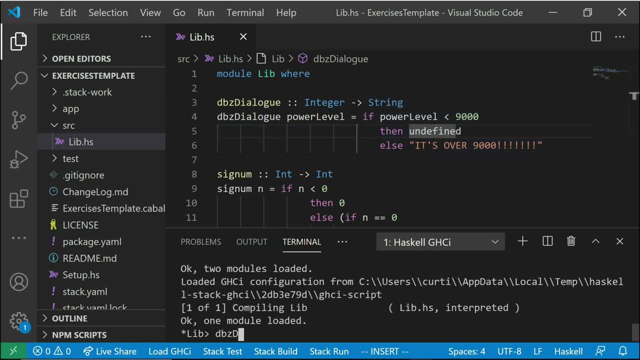 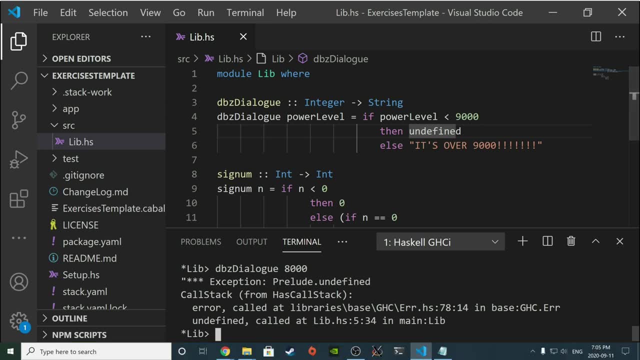 and we call dbzDialog 8,000.. Okay, you see, you get exception: prelude: undefined. Now, this isn't very good. This is why we should never, ever, ever write- just write undefined, because, let's say, you're trying to fix your program. 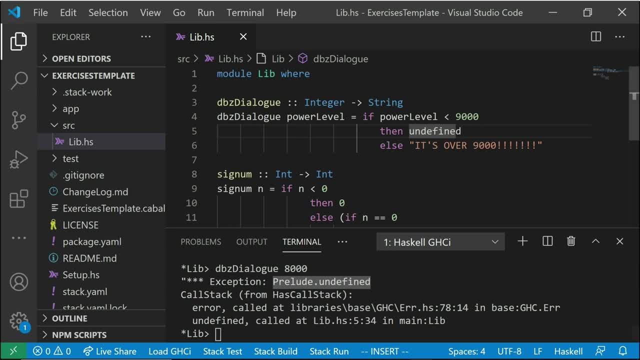 and you're trying to find out like, oh, where did this happen? And you have multiple undefineds written all throughout your program. It's gonna be very, very difficult to figure out what is going on. So what you should do instead. 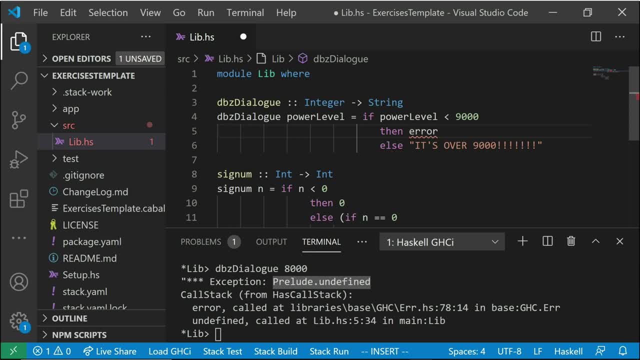 is you should use the error function, And the error function takes a string and this string will get outputted instead of just this preludeundefined. So never use undefined, always use this error function And you could write something like: this program is too lame to keep running. 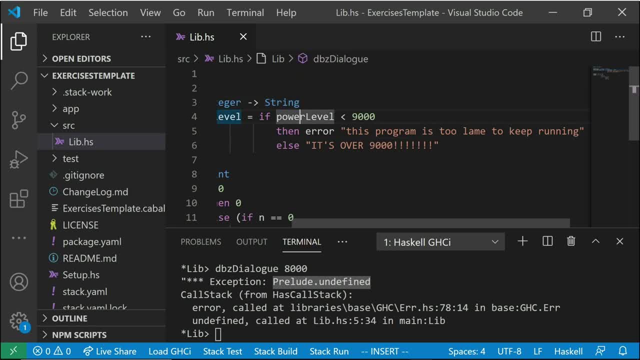 Okay, it should be a specific error message to what's going on So that it's easy to track down. So now, if we reload this in the GHCI, okay, make sure your file is saved first and reload, And then we run this again. 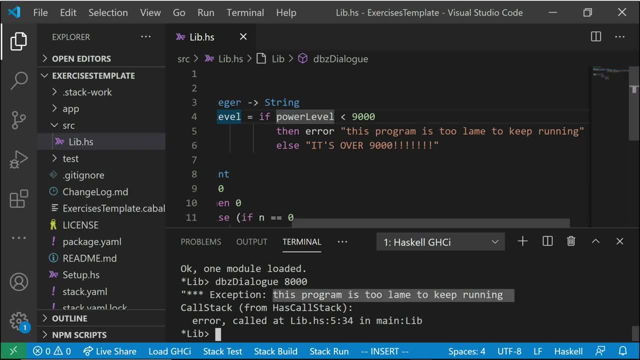 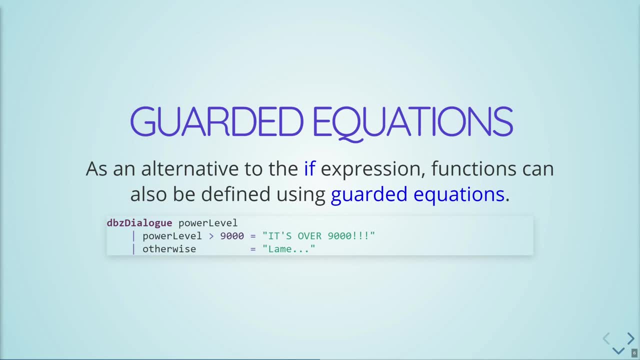 See now it says exception and it gives whatever I put in that string here As an alternative to if expressions, we can use guarded equations. So this has a syntax that uses this, this vertical bar, before you define the function. So usually we write something like: 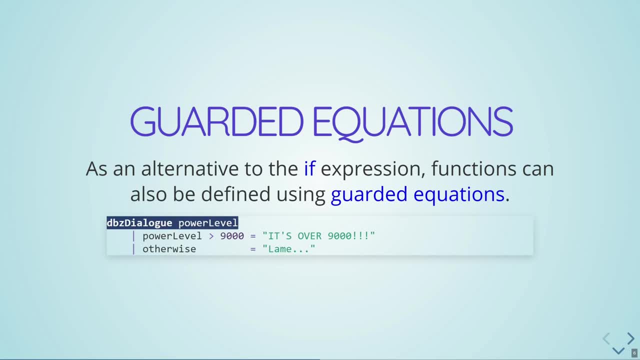 our function is equal to this expression. And at that point we might write: if something something, then this, else this, With guarded equations. what we do is we say our function and then we write: these guards, okay, these vertical bars. 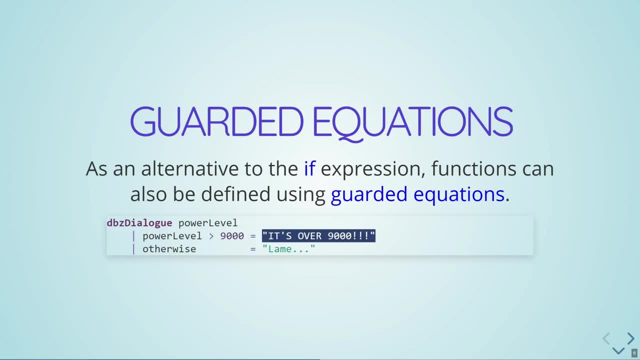 and we put our Boolean expressions and we say what our function is equal to, what the definition of our function is equal to, based on these um Boolean expressions. Okay, And you have a default Boolean expression here, Otherwise, otherwise always evaluates to true. 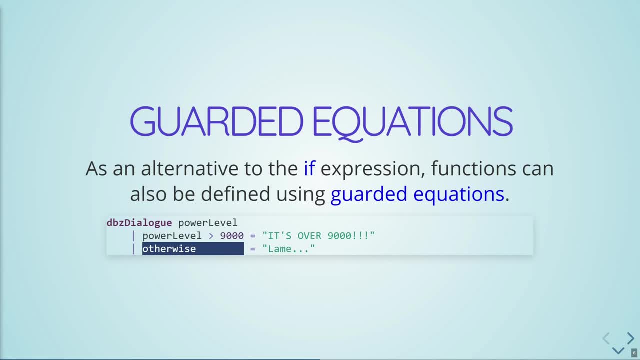 So you should always put it whenever you have a series of guarded expressions, otherwise should always be the last thing here. Now. a note about guard equations is there's never really a reason that you would have to use them instead of an if expression. 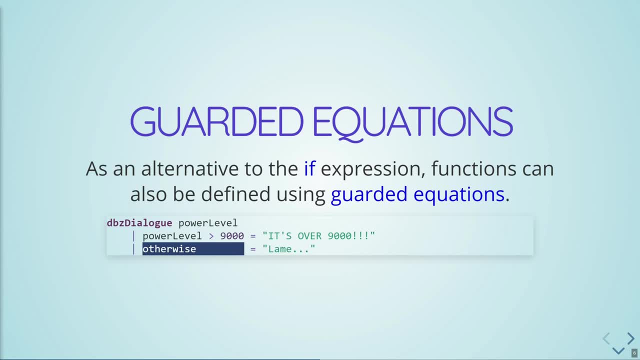 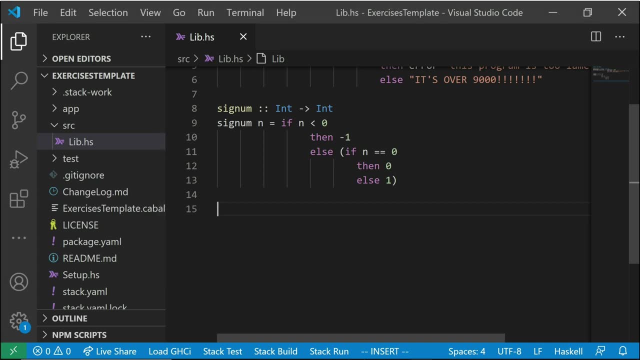 They're completely interchangeable. It just looks nicer. It's just something that you can do. It's sometimes a nicer way to write out your code. So let's go back to our code here and let's try and create an improved version of our signum function called signum two. 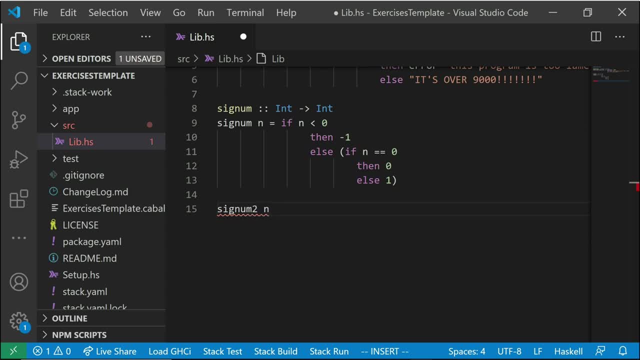 And this is actually going to be the exact same function. It's not going to be improved in any way, except that it's going to be more readable. So, instead of just saying equals here, what we're going to do is we're going to put a new line. 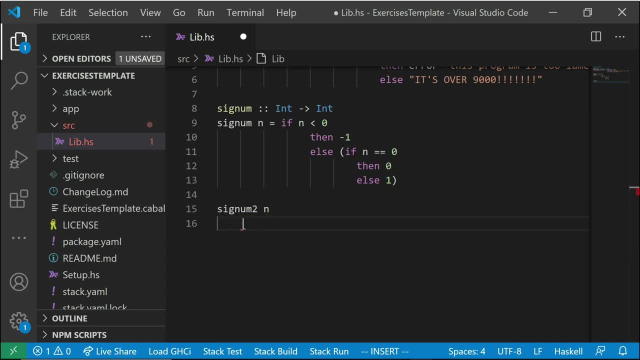 indent and put our vertical bar and we'll test our first condition of: is n smaller than zero? And if it is smaller than zero, then what the function is going to be equal to is negative. one New line. make sure this lines up. 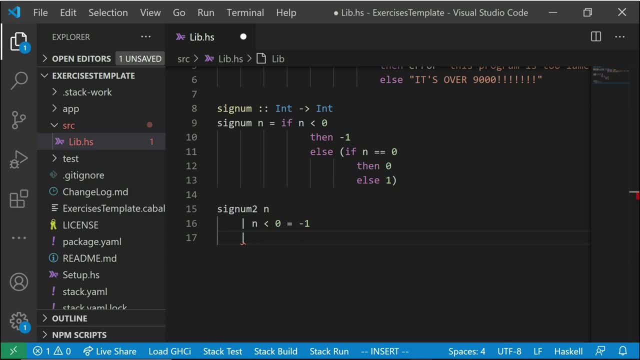 Vertical bar. they should both line up Indentation matters. N is equal to zero. Okay, this is our second condition. And if it is equal to zero, then the function is going to be equal to zero, And then the third scenario is going to be: 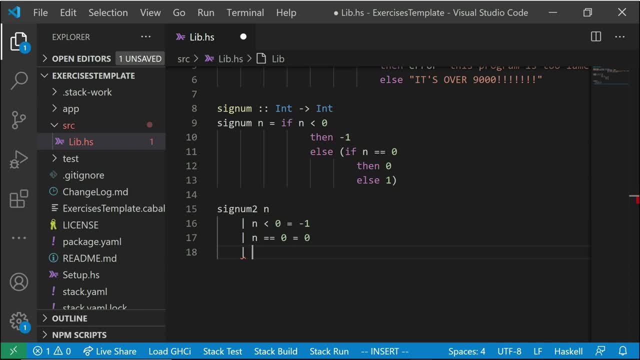 if n is bigger than zero. But a better way to do this- to make sure that we cover every single scenario- is just to write otherwise, which is actually the same thing as just writing true, But otherwise is a bit more readable. It's just kind of nice to read. 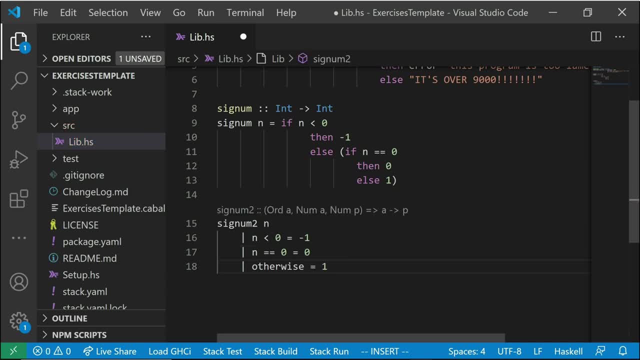 So otherwise equals one And comparing these two functions you'll see they're the same thing, They'll work the same way, but this function is a decent bit more readable than this function, Another construct that could be used as a condition, although this one is actually far more powerful. 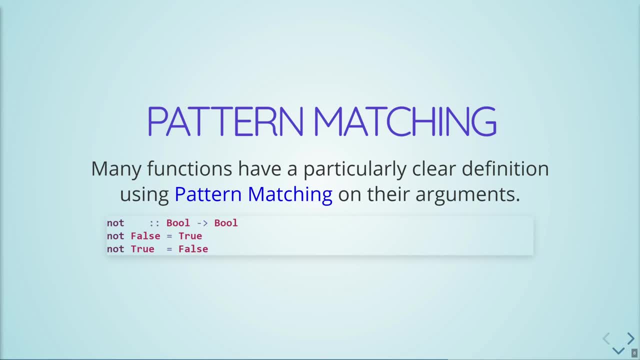 than just conditionals is pattern matching. So pattern matching allows you to write values in place of where you would usually just put your parameters. so your argument variable- You actually write the real value there and then you make multiple definitions of the function. 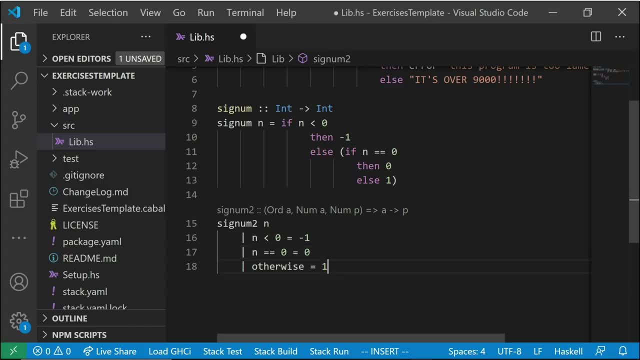 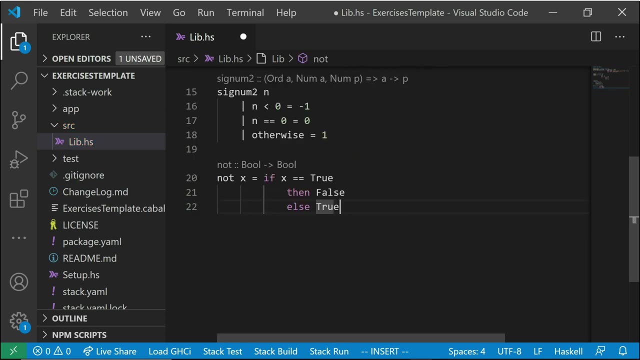 So consider, not as an example, Not takes a parameter, a Boolean parameter. we call it x, okay, And if x is true, then it returns false, Otherwise it returns true. So it's kind of returning the opposite of whatever its input is. 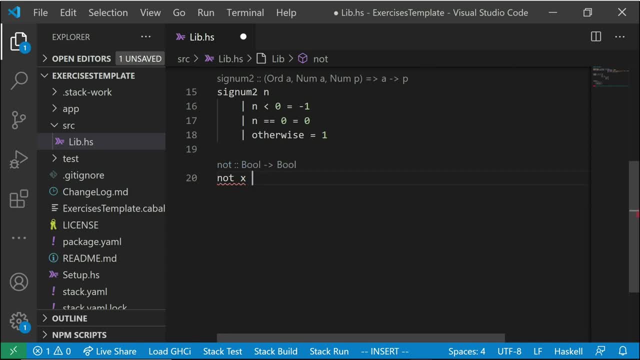 So this is one way we could have written, not Could write it another way, with guards. Or we could write a third way, with pattern matching. So the idea with pattern matching is, instead of writing x here and then the function definition, we would write the value that we're matching x to. 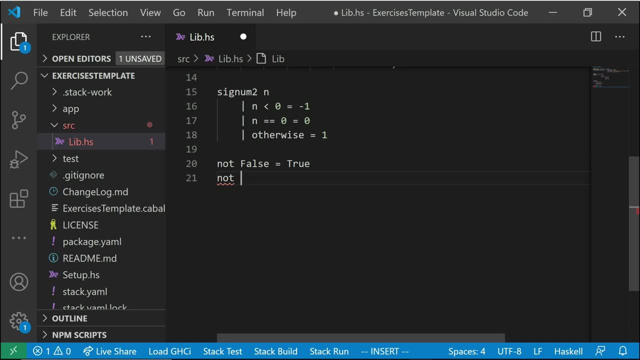 and then the function definition, and then we just keep defining the function again with the value we want to match to, and then we can get to the point where we want the function to match to. So we have, in this sense, we have, like multiple definitions of our function based on the value of its input. 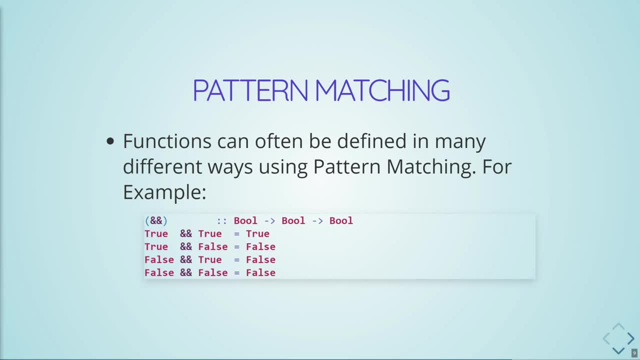 You go about pattern matching in a variety of different ways. consider the and function so a logical and returns true if, and only if, Both of its inputs are true. So it takes two inputs and you're basically saying this and this, so only if both things are true. 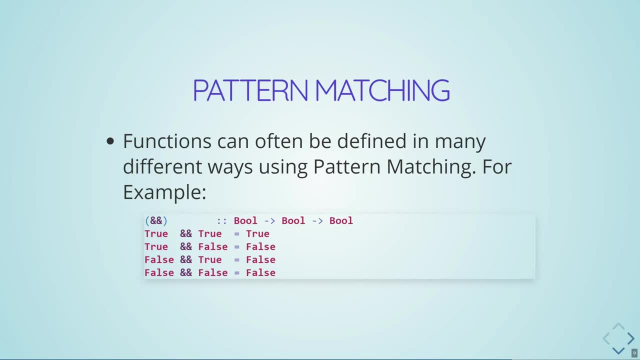 Is this going to return? true, So we go about defining this by writing out every single scenario for both inputs And pattern match on them. Okay, so we end up because there's two inputs and each of those inputs can have two separate values. There's going to be four different scenarios here. 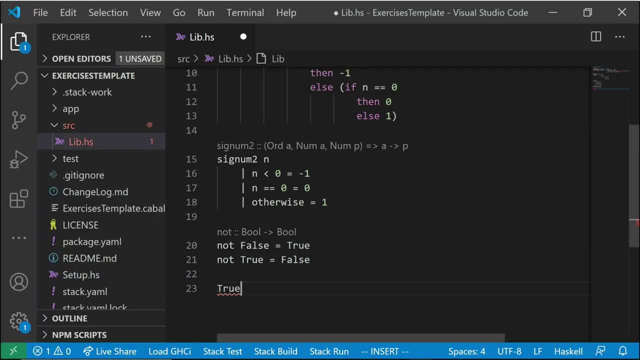 Now the nicer way we could write the and function Is: well, pattern match on the First argument and we'll pattern match to true, and then for the second argument, we'll leave it as a variable. We won't pattern match it, and the reason we'll do this is if the first argument is true. 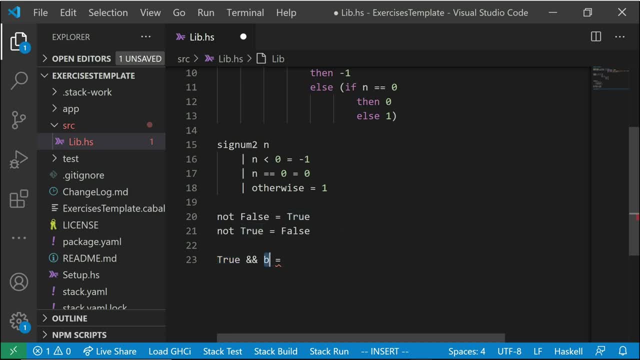 Then the result of this is going to depend completely on the second argument. So if the second argument is true, we'll have true and true, which is true, And if the second argument is false, we'll have true and false, which is false. So we just return b and it's in its stead here. So the first argument is true.